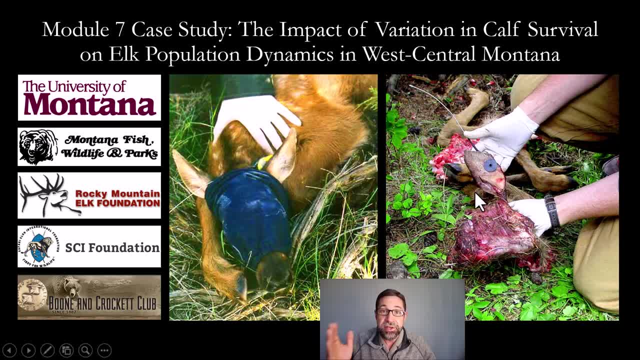 determine cause specific mortality rates of these elk calves in this elk herd that showed declining recruitment. Really proud of the work that we did here because this work really shed some light on truly driving inter-annual changes in population abundances of elk herds that are observed by 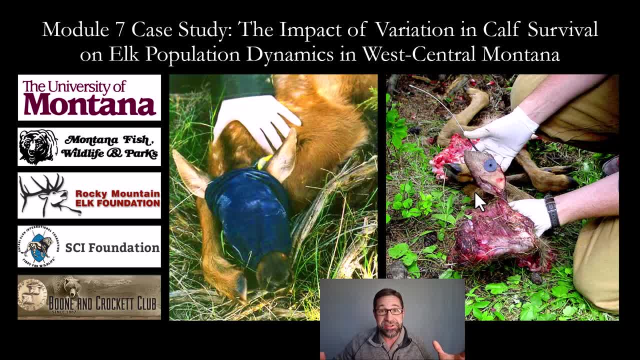 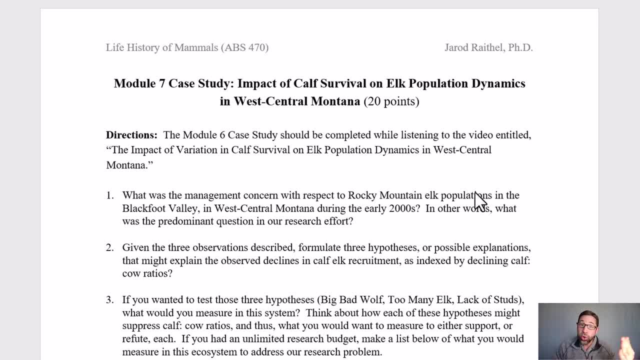 wildlife managers in the western United States, So hopefully you'll find it enjoyable. So, just like last time, there's a case study in a Word document that's in Canvas. I'd ask that you open that now, if you haven't done so, and please follow along through this presentation and just go ahead and 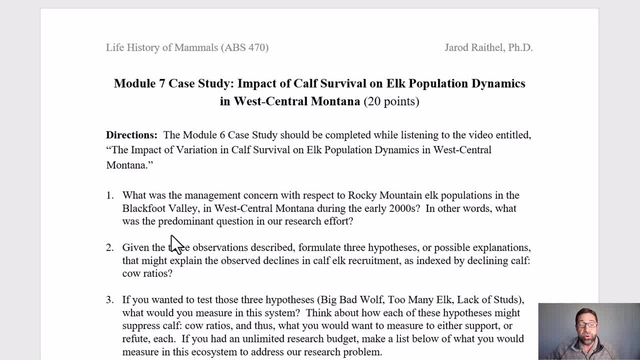 really input your answers into the Word doc to be uploaded to Canvas. So some of these questions are somewhat subjective. There are no right or wrong answers- A lot of it, or there's a handful of questions about experimental design as well as interpretation. So don't sweat it if what you 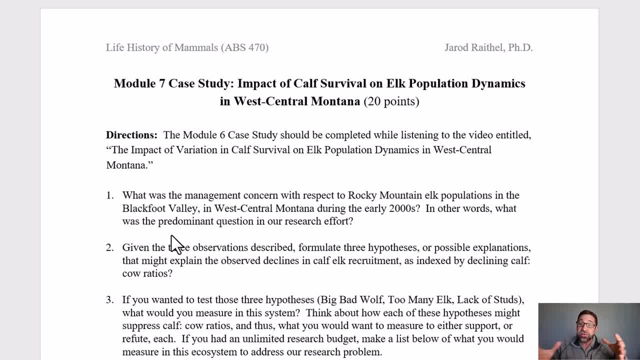 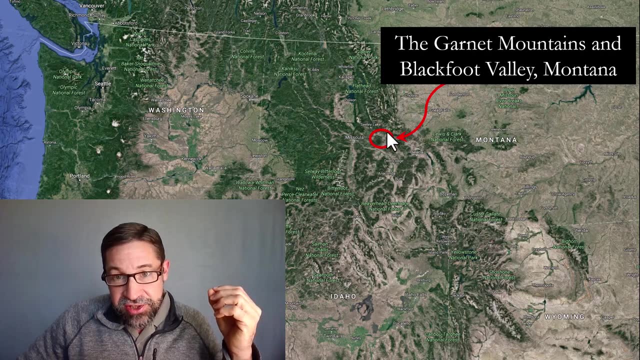 choose to measure or how you interpret these data are different from the way we did, So this is based on your participation And your engagement, as well as providing me some thoughtful answers. Okay, so we were located. Our study site was in Hunting District 292, which was about 40 miles east of Missoula, Montana. So this 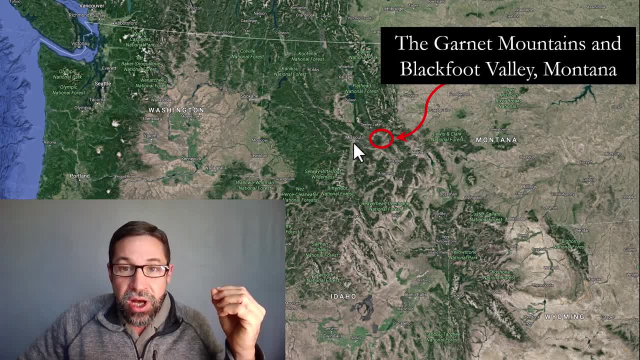 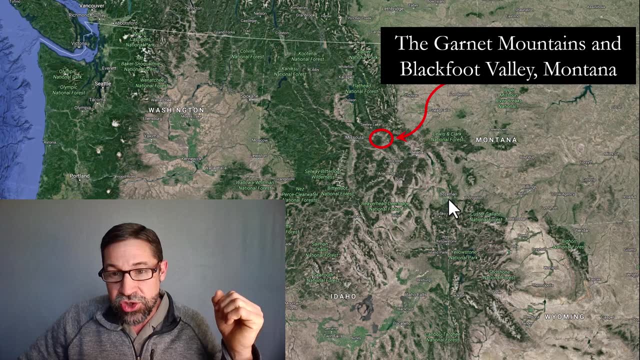 is West Central Montana here. This is Missoula, This is where the University of Montana is. You guys may be familiar with Bozeman, which is down here, just north of Yellowstone National Park, which is here, But we were in the Blackfoot Valley so the Blackfoot River runs right through here, as well as the Garnet. 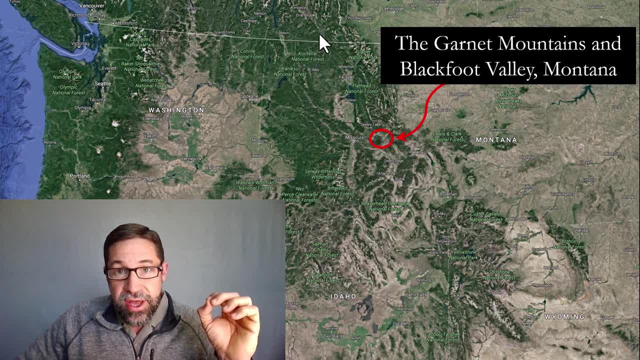 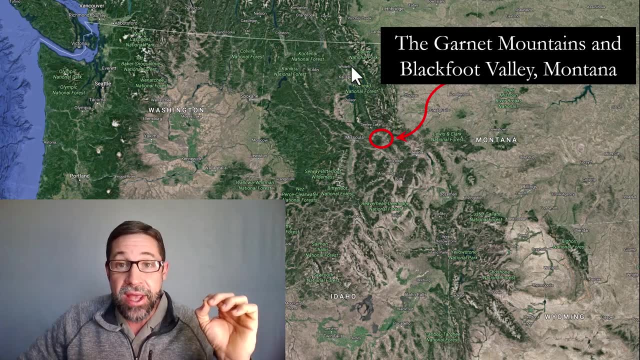 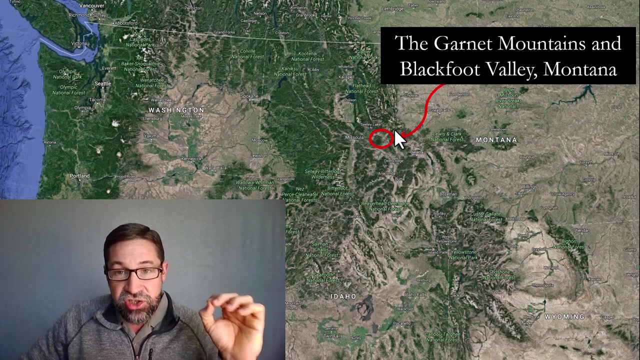 Mountains here. So I would point out that this represents the largest contiguous track of wilderness in the lower 48. So this is Glacier National Park and it's going to tie into the Bob Marshall Wilderness which runs the way down past Seeley Lake to Ovando, at the edge of our study site. so this 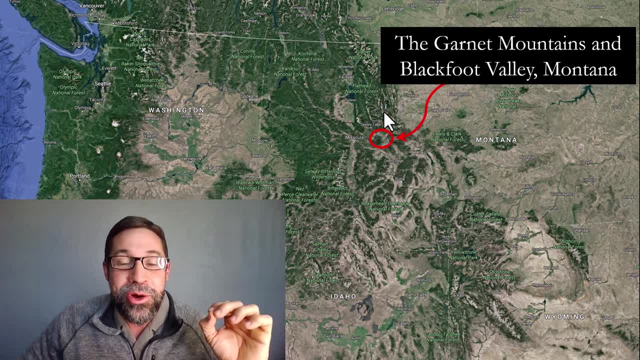 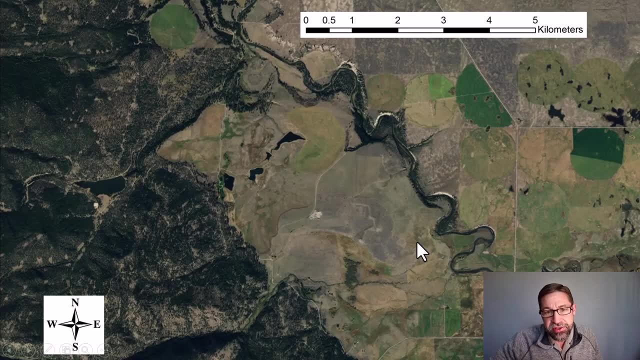 represents a corridor for those recolonizing wolves, which I'll discuss here in just a second. however, if we zoom in for closer inspection, this is the northeastern corner of our study site. even though we're on the edge of this very vast, contiguous wilderness area, our study site still represents a heavily 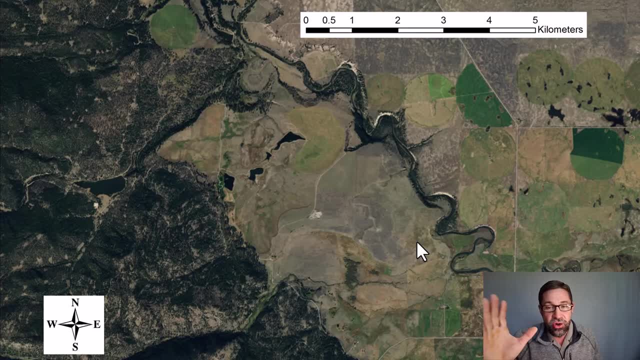 modified landscape, so this is still dominated by human activity. so this is the winter range here, the low country along the Blackfoot River, and you can see that it's almost entirely been converted to agriculture. so this green, these bright green areas, these are alfalfa pivots. they're irrigated. 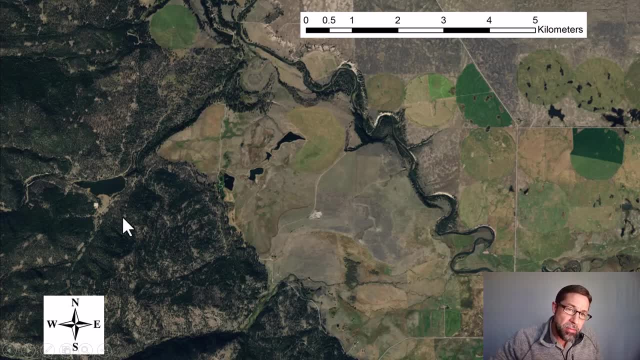 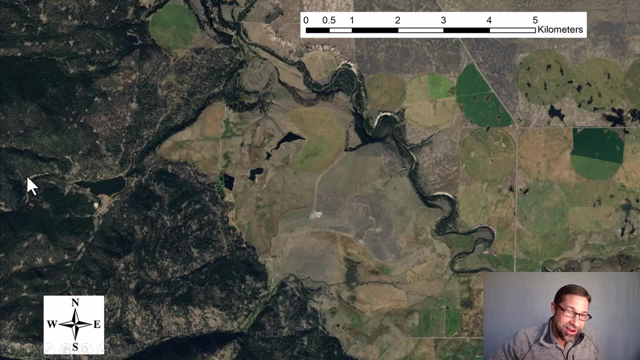 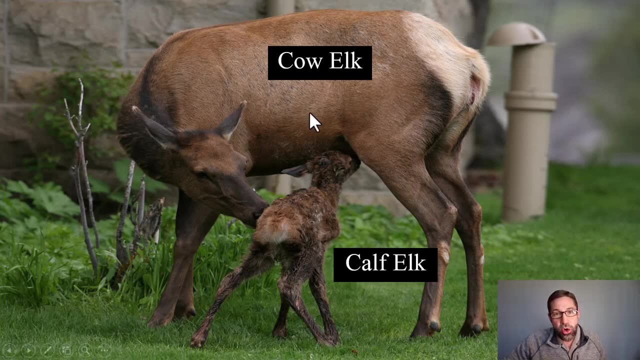 clear cuts like you see here, as well as lots of logging roads. okay, before we get too deep into this, some basic elk terminology. so hunters and wildlife managers are going to refer to female elk as cows. so this is a cow elk elk, And then this is a calf elk. So it's considered a calf from the moment it hits. 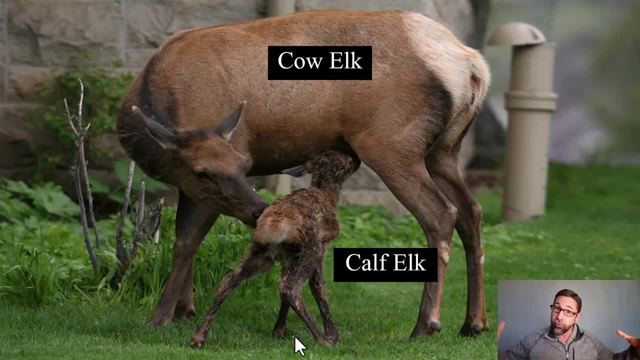 the ground, like you see here, all the way up until its first birthday, beyond which we then call it a yearling, as we discussed when we discussed age classes in our last lecture. You can also further subdivide that first year of the calf's life up into the: 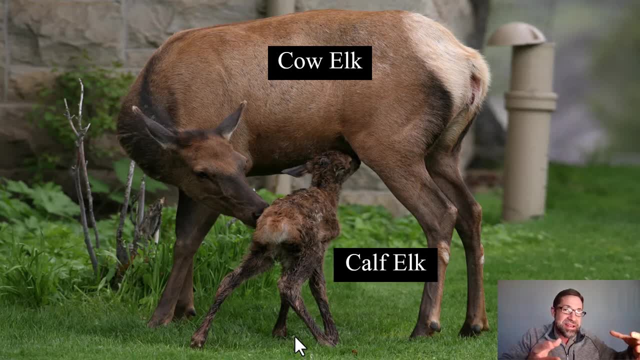 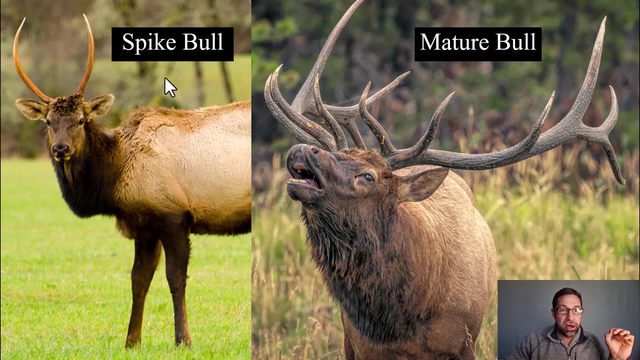 neonatal period, which is typically about 90 days, those first three months getting us through the summer period, and then the juvenile period, which is typically the fall and the winter. Similarly, we refer to immature males as spike bulls. Remember Cervus alaphis. 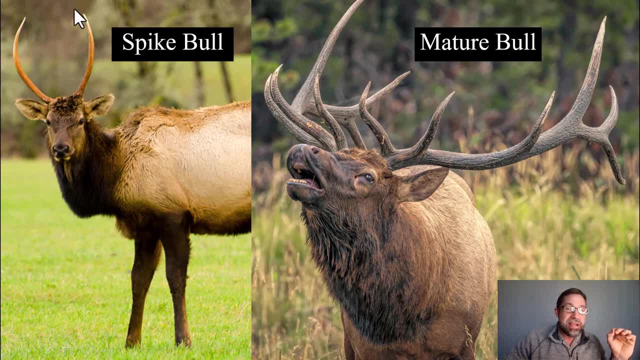 or Cervus canadensis, the elk, the wapiti, the red deer. if you're in Europe, They have antlers, so they grow antlers every year. They don't have horns, which we'll talk about when we talk about this order here later. 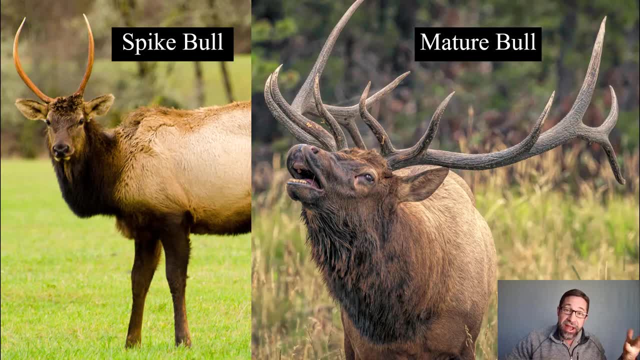 Under this module. so their first set of antlers that they grow typically doesn't have any branches, It's just a single spike. So this spike bull is likely one and a half years old, where this is clearly a mature bull, often referred to as a branch antlered bull. 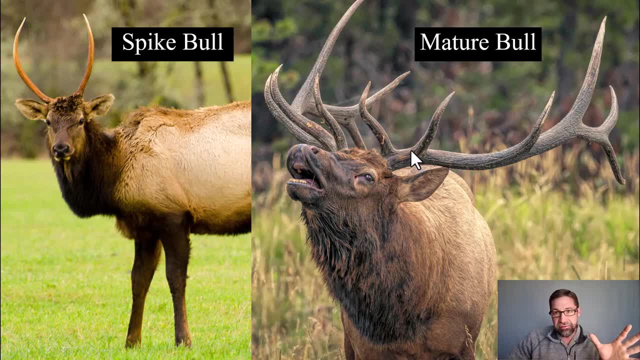 So they're going to get their first branch antlers, usually at two and a half, but this is a prime aged bull, So this is referred to as a six by six: One, two, three, four, five, six tines on the antlers, Six on each side is six by six. 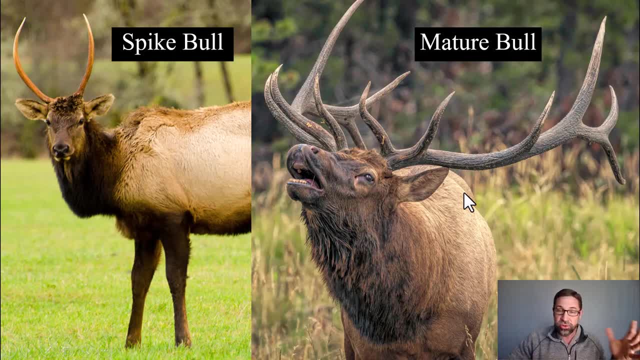 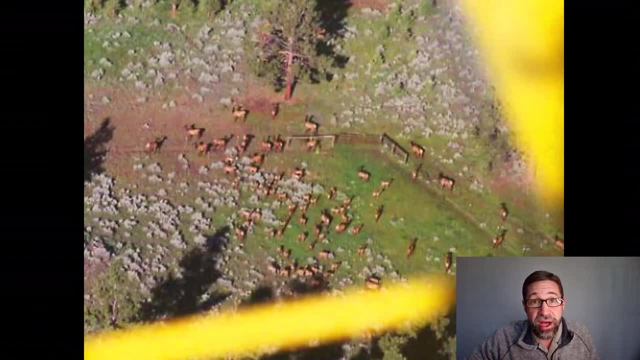 So this is a prime aged male. so it's minimum six, seven years old. It may be as old as 10.. Every spring across the western United States, wildlife managers for various fish and game agencies are going to get up into little fixed wing aircraft and they're going to systematically. 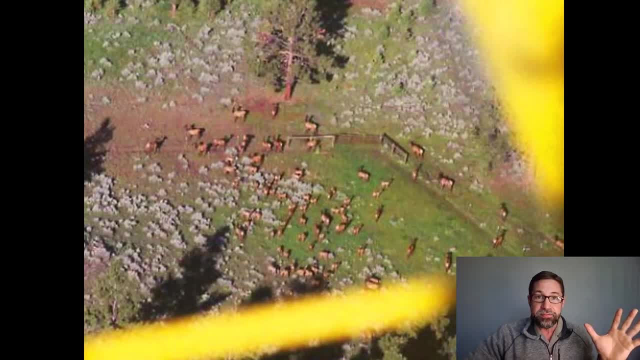 serve your ungulate herds. So these are typically called spring green-up surveys and they're a measure of recruitment of elk calves that were born the following year, that are about to be recruited into the population as yearlings. So I did these spring green-up surveys between 2002 and 2005 on. 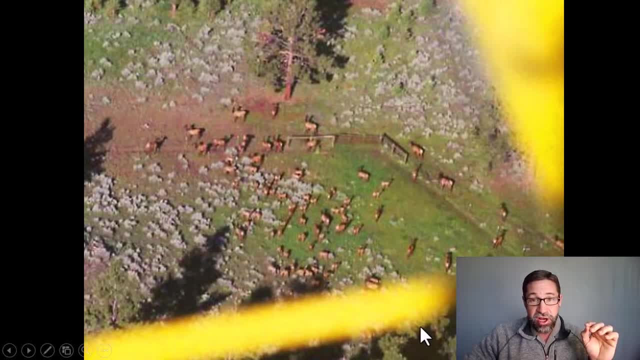 this hunting district for Montana Fish, Wildlife and Parks. This is a photograph that I took. this photo, Like all photos in this presentation, were shot using film. This is before digital cameras were widely available, so that's why it's a little grainy. It's been scanned in. 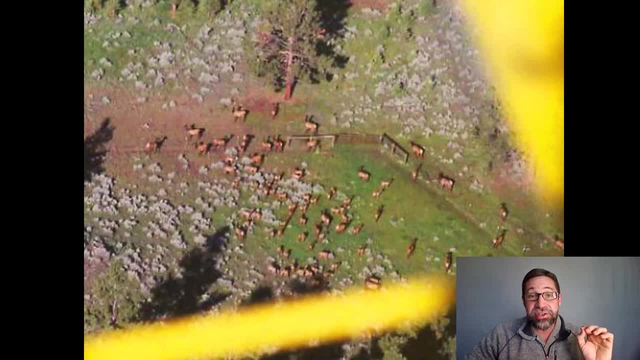 But you get up in these tiny little fixed wing aircraft. So this is a super cub. It's just a little two-seater. My pilot was the famous Roger Stradley, So Roger's flying the plane and I'm in the back and the goal is to count and classify the elk herd. What do I mean by that? 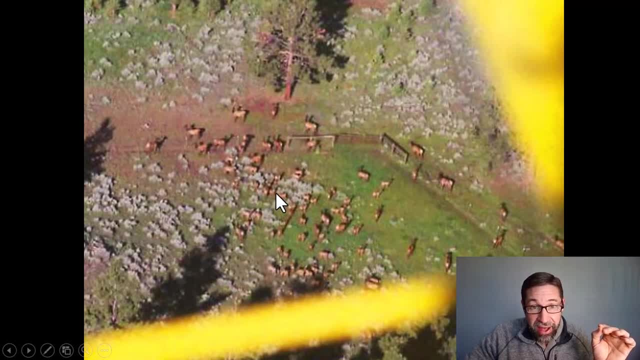 This is a cow cow, cow, calf, calf, calf, and so what you're going to do is you're going to generate this metric called a calf-cow ratio. So managers want to know how many calves are produced per hundred cows, because it's a measure of recruitment, The number of young that are going to be recruited into the. breeding age population. The number of young that are going to be recruited into the breeding age population. The number of young that are going to be recruited into the breeding age population. The cow-cow generation. The man of群십 is going to get called in for the caravel measure of seven hours per carnage. 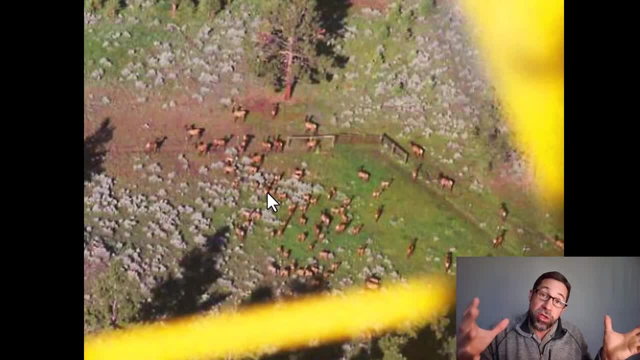 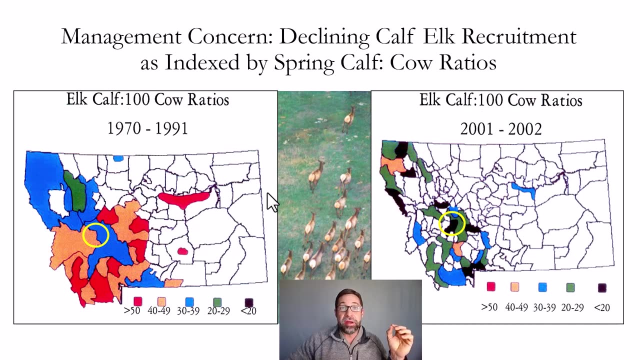 the calf cow ratio. you can also generate bull cow ratios and I'll be discussing both of those in this presentation, but let's start with calf cow ratios. so the major management concern, the reason why we were funded to do this work was because of declining spring green up calf cow. 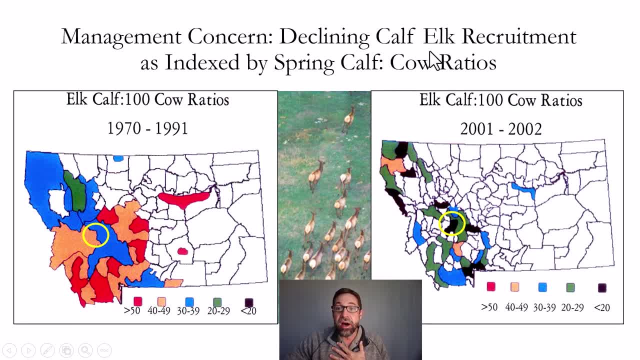 ratios, which again are an index of calf elk recruitment and we know recruitment is a measure of the young that are about to enter the breeding age population. so I've got our study site circled in yellow but you can look at trends across all of Western Montana. so this is average. 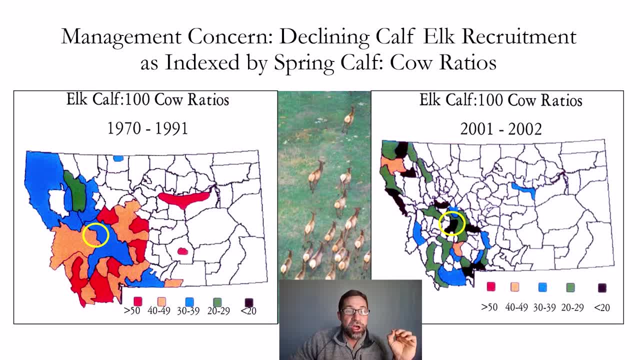 calf per hundred cow ratios between 1970 and 1991, so a 21 year period, and you can see in many places over 50 calves were counted per hundred cows. on our study site it's between 30 and 50 calves produced per hundred cows. okay. however, when I start this work in 2002, calf cow 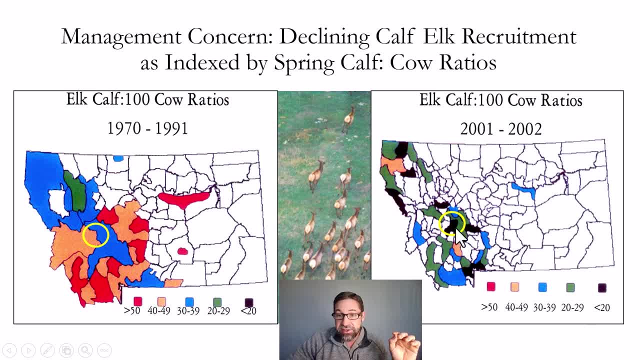 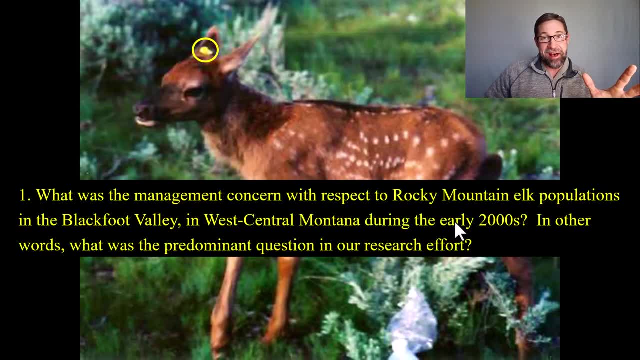 ratios on our study site have declined to less than 20 calves produced per 100 cows. so the first question, which was: how many cows do you rejected here in receiver degree we found at a community question I have for you on your case study, is: what was the management concern? What were managers? 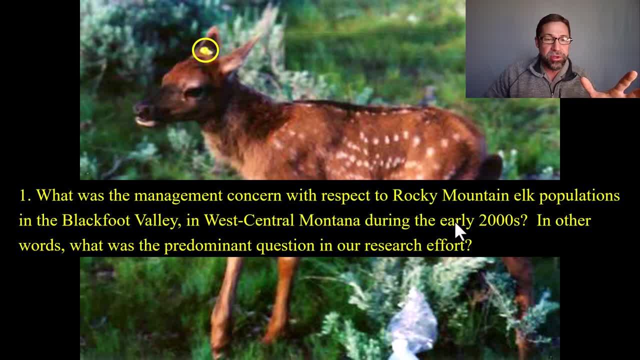 worried about with respect to Rocky Mountain elk populations in the Blackfoot Valley in west central Montana during the early 2000s. In other words, what was the predominant question in our research effort? Hopefully you picked that up. So to begin with I needed to put these declines. 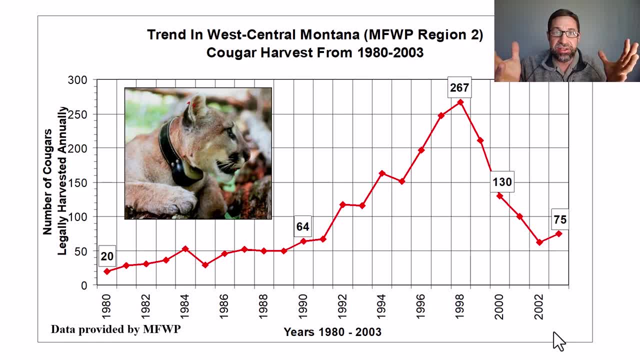 in calf elk recruitment into context. What else was going on in the system? What else were we observing at this time? Well, one of the things that jumped out at me right off the bat was the increase in mountain lion harvest in region two, which is west central Montana, which peaked at 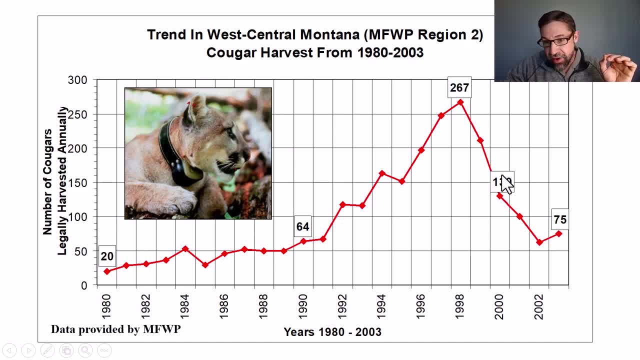 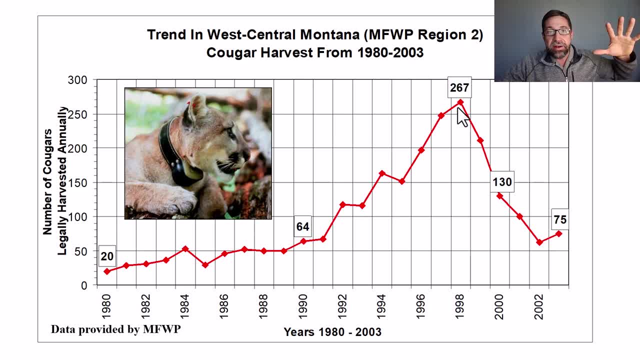 I learned that lions may have been over harvested and mountain lion populations were suppressed, reflected in these lower harvest rates. But I learned a valuable lesson in talking to the management biologist. It was actually the houndsmen- the lion hunters in 1998 that petitioned. 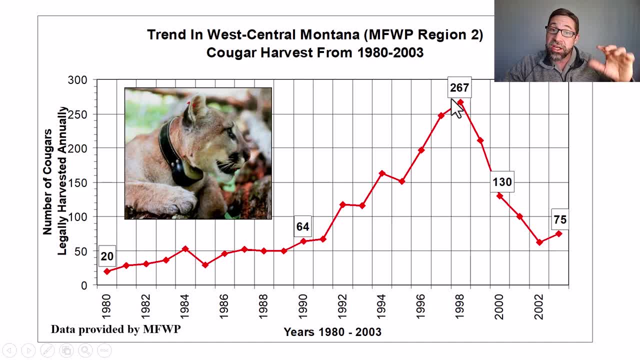 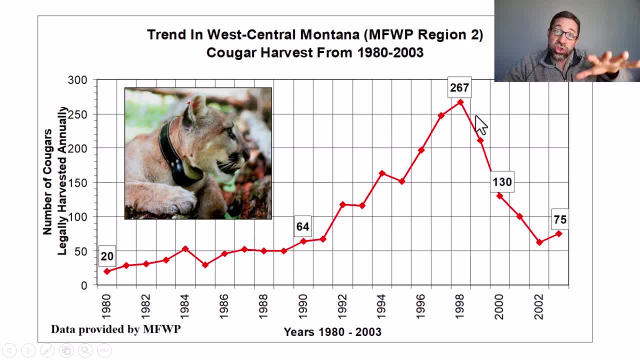 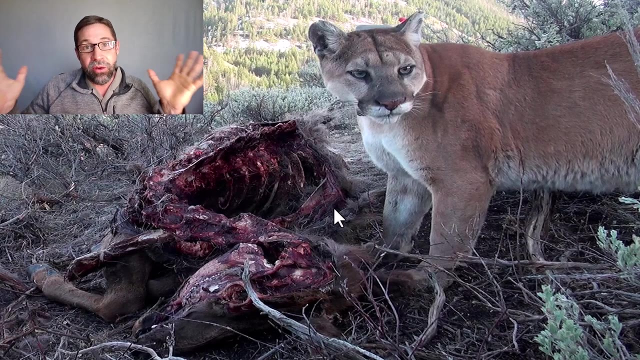 during this period, Montana Fish, Wildlife and Parks was restricting mountain lion harvest. they were reducing the number of permits issued, So less lions were being harvested. So what that meant was there were more mountain lions in the system in the early 2000s than there had been historically. Of course, we know mountain lions are a primary predator on cats and they 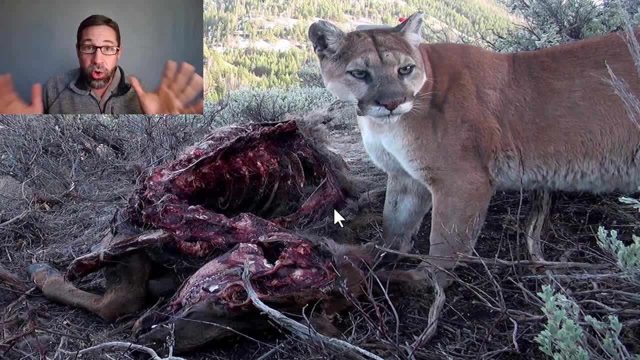 elk. so I talked to you about the work that I collaborated with out of South Dakota when we talked about the fundamental versus the realized niche and we established, at least in the Black Hills, that mountain lions can exhibit top-down regulation suppressing elk calf herds just by their sheer predation rate. 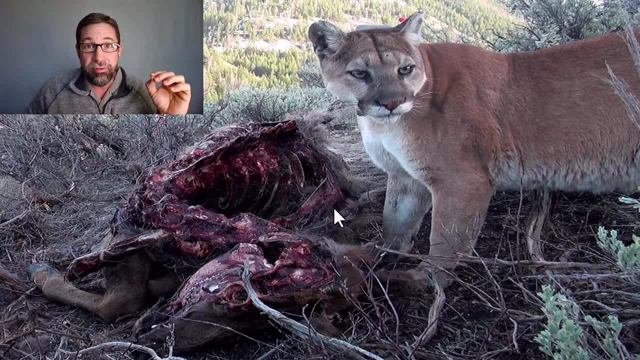 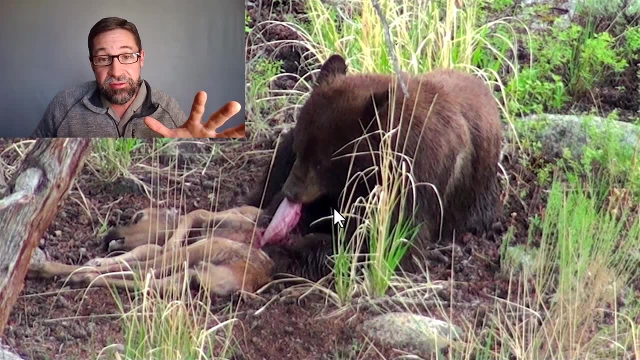 on the calves. so this is a significant predator of elk. we also know from bear hair snare studies that Montana Fish Wildlife Parks had done and other folks had been up to the USGS that both black and grizzly bear populations were also increasing at this time in west central Montana and bears were also thought to. 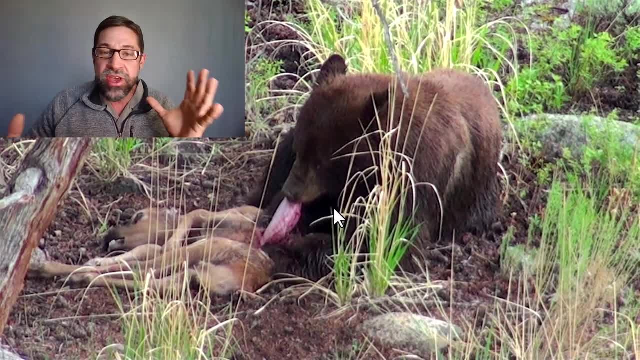 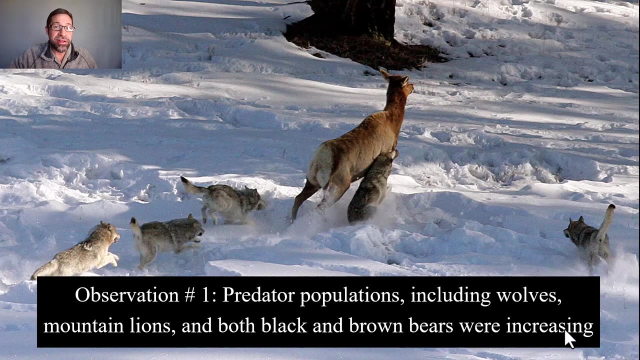 be a predator on calf elk, although we didn't know the extent to which bears would play in this. in this system, and then perhaps of greatest concern, at least to sportsman's groups, was the recolonizing gray wolves. so wolves were moving into the area, into the Blackfoot Valley, in the early 2000s. 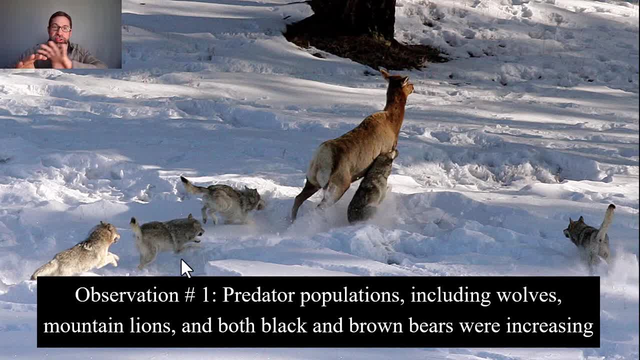 important to note. these were not likely wolves that were descendant from the wolves that had been translocated into yellow stone national park in the mid 90s. these wolves probably recolonized on their own from Banff National Park down through Glacier and the Bob Marshall. 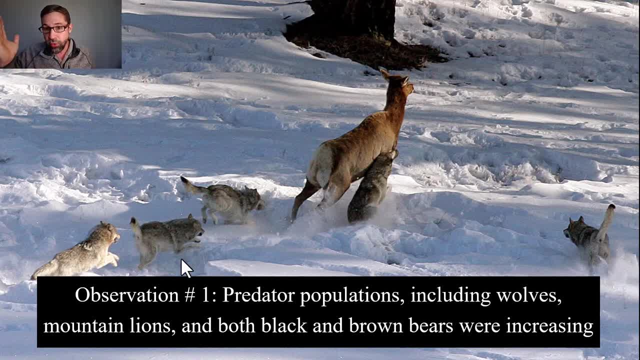 Wilderness. but regardless of how they got there, wolves were moving into the system. so within the Garnett Mountains and the Blackfoot Valley on our study site, we could confidently say that mountain lion, grizzly bear, black bear and gray wolf population were down to around 80,000. Amazing. 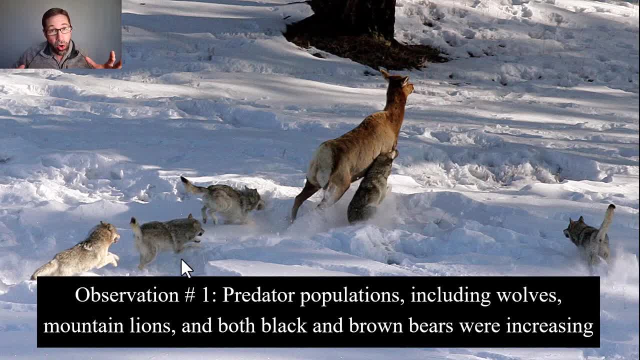 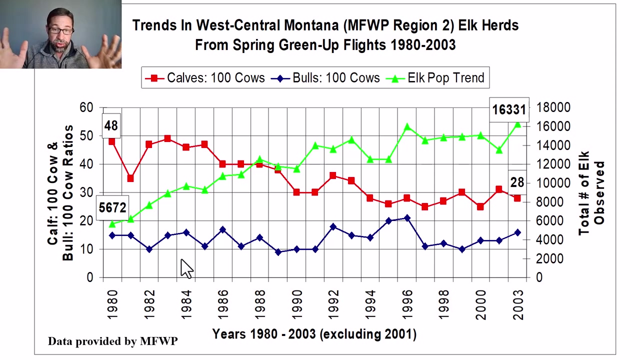 of predators on elk were all increasing. So was calf elk recruitment being regulated by top-down forces? Was it the predators that was limiting the number of calves that were being recruited in this elk herd? The second big observation that I made was based on looking at the flight data. So these are spring greenup. 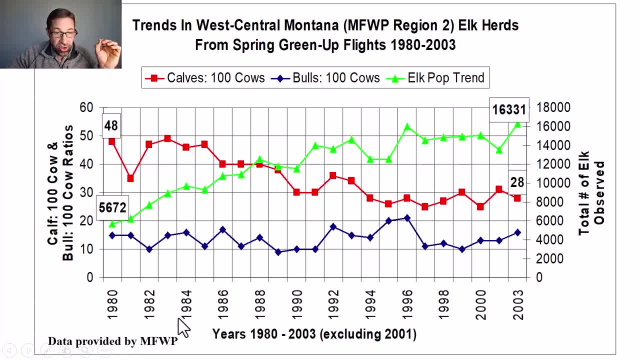 flights from 1980 to 2003.. Time is on the x-axis, so the calf and bull cow ratios are here on the y-axis. on the left-hand side, We'll start with this red line. This is the proportion of calves counted on spring greenup flights. 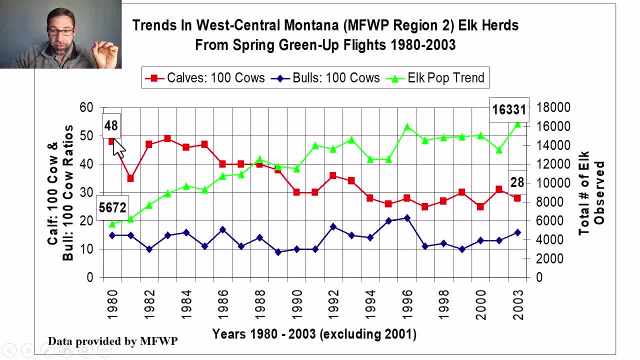 in Region 2, West Central Montana from 1980 to 2003.. You can see we've got 48 calves per hundred cows in 1980.. You can see we've got 48 calves per hundred cows in 1980.. 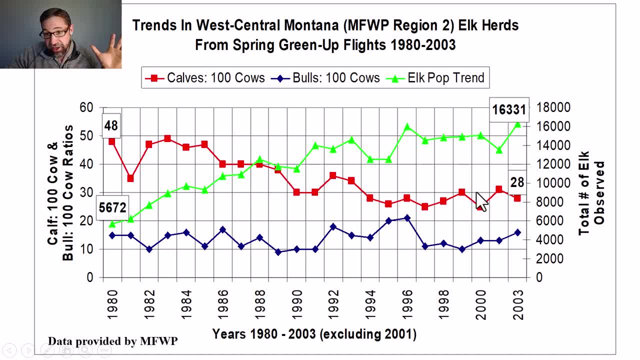 You can see we've got 48 calves per hundred cows in 1980.. then that declines. we see this steady decline all the way to the 2000s and I did several of these surveys and we were at mid-20s calves per hundred cows, so essentially half of the calf. 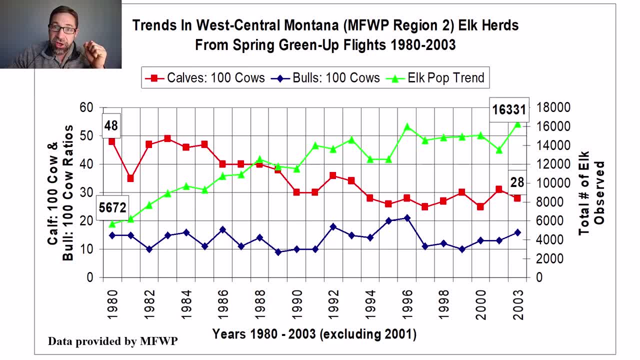 recruitment that we'd had two decades before. but the other thing I want you to note here is this green line. so this green line is total number of elk observed on green up flights. so this is an index of total abundance. the same. so the pilots and the managers are flying the same areas year in. 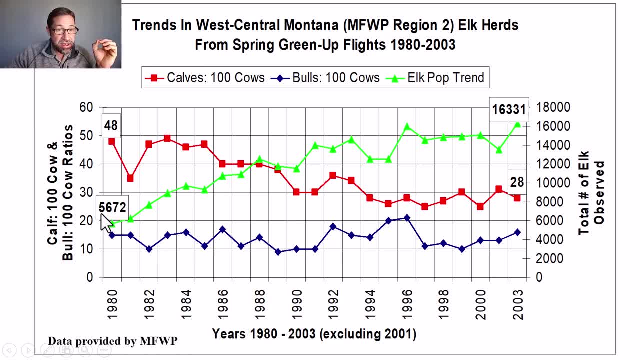 and year out for consistency's sake. in 1980 5672 elk were counted, by 2003 16 331 elk. so we see a tripling of elk abundance in region two during this time period. and we know that elk are a slow tempo k selected species. so when that population abundance gets over a certain size, 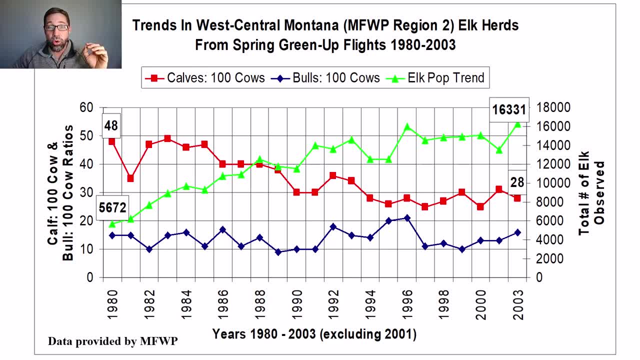 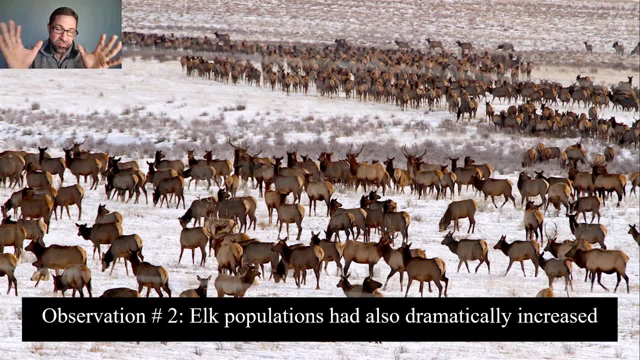 we have that inflection point and population growth is going to decline. okay, so the second observation that we make is that elk populations have dramatically increased. so maybe it wasn't the predators at all, maybe it was bottom up regulation, so maybe the elk herds had gotten so dense. 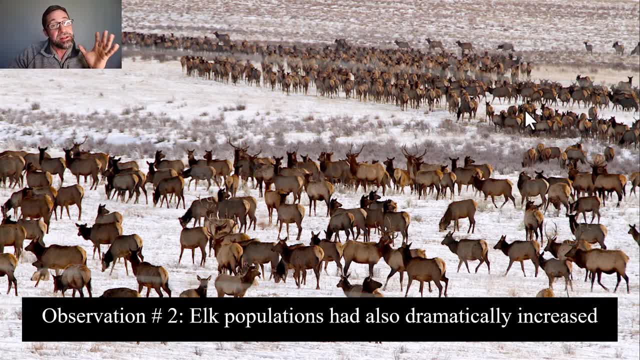 that vital rates were beginning to be impacted. maybe less yearlings were getting pregnant. maybe prime aged adult cow elk had lower pregnancy rates. maybe on elk winter range you have high densities of elk and you don't have a lot of forage. who's going to lose out? it's going to be. 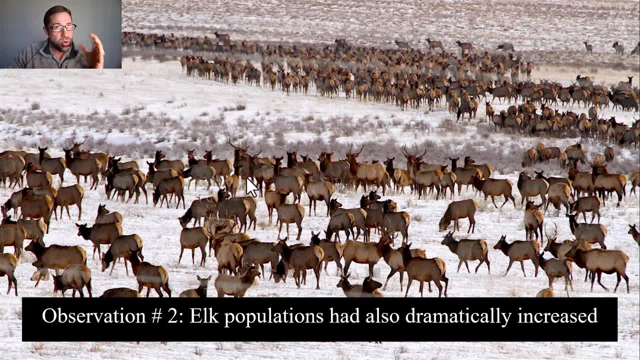 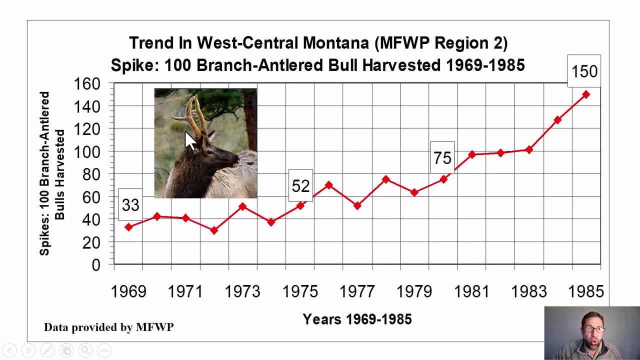 early or early calfs. they're the most likely to not make it through those lean months. and if they don't make it through, if calf survival drops during the winter, then so does calf recruitment. and then the third trend that i want to bring to your attention is the proportion of spike bulls. 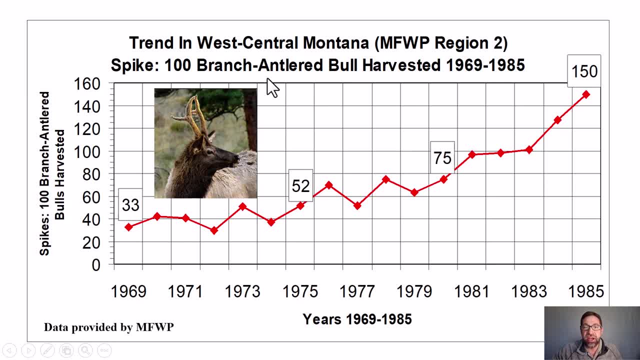 harvested, relative to every 100 branch antlered bulls harvested, and the data was available from the late 1960s, only up to the 1980s. but the trend around the United States is that k-9 and k-3 are the most likely to lose out over the winter period when the bulls are moving down. there's a high chance. 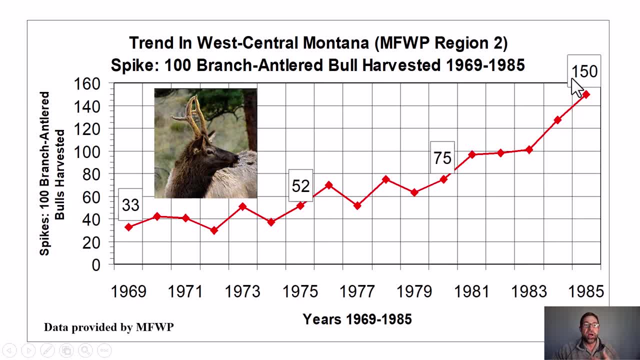 was clear, hunters were harvesting a greater proportion of these young, immature bulls relative to prime aged mature bulls, and that wasn't via preference. that wasn't because they were trying to go after spikes. that doesn't make for a very good trophy right, so most hunters want to harvest that big. 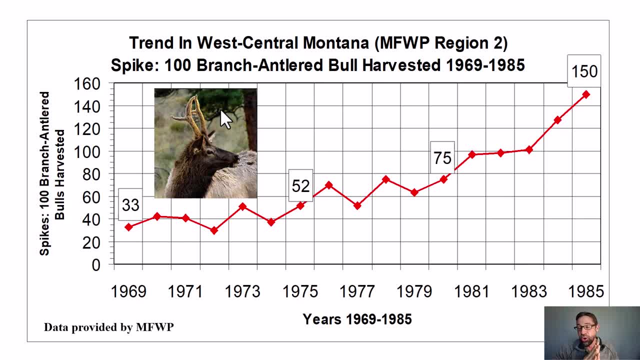 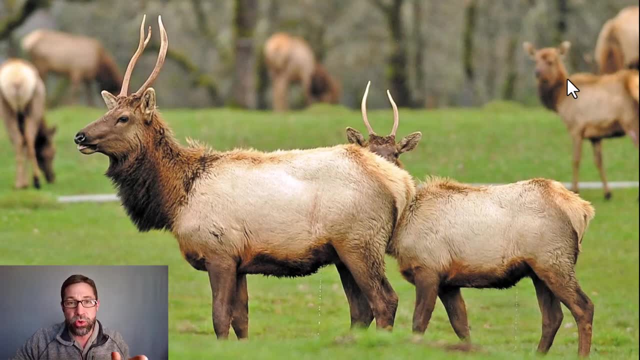 prime aged mature branch antlered bull. however, they end up harvesting spikes, because this is a reflection of what is out there. oh, the concern was, perhaps these herds had a very low proportion of prime age branch antlered bulls. well, how might this impact recruitment? okay, so follow me. so these spike bulls, these, 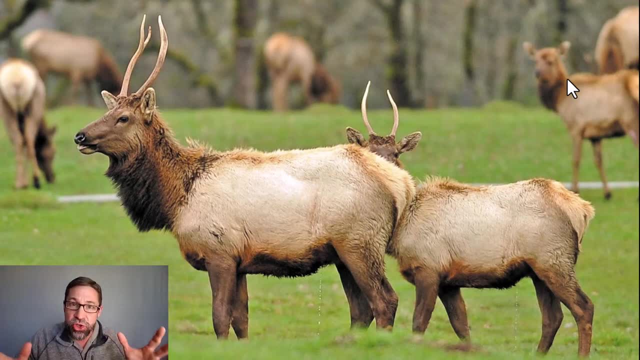 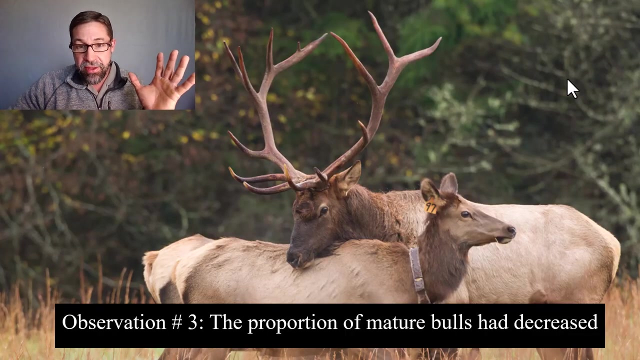 immature bulls. they don't really know what to do during the rut. they don't have a lot of life experience. so, remember, the cow elk are going to all go into estrus at the same time. in the fall, it's called the rut. okay, when they go into the rut, remember these are polygynous species, so 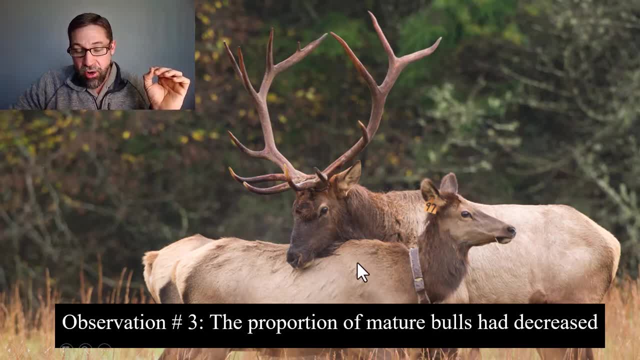 you have one prime aged bull with this harem of cows and he is going to breed all of those cows in a short amount of time. you so, in doing so, the gestation period is relatively fixed. so as we move into the spring, all of those cows that became pregnant at the same time they're now. 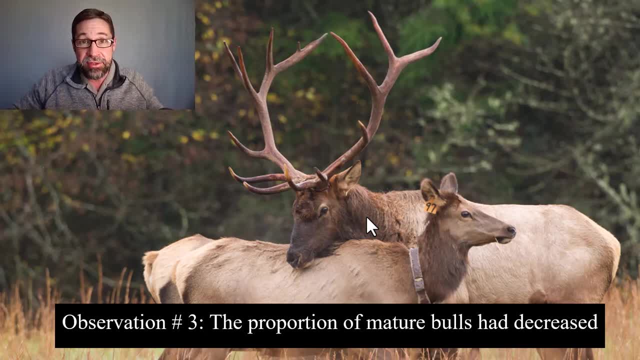 all going to drop their calves at the same time. they're going to have a very synchronized calving period, and this is a strategy. the idea is to satiate the predators. so you remember the type 2 functional response of predators. so as the density of the prey goes up, the 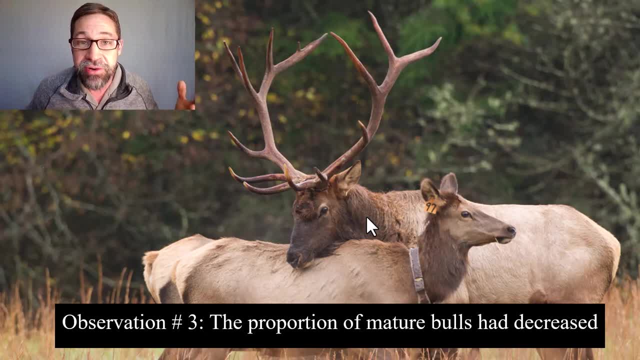 predation rate actually levels off. why? because the predators get full. they can't eat any more prey. so the idea here with this synchronized calving period is to flood the system with calves, and then the predators are only going to be able to kill so many of them, and the majority of those calves make it. through that dangerous neonatal period. However, if there aren't enough prime-aged mature bulls in the system, if you only have these immature spikes, if they don't breed the cow elk when she first goes into estrus and she ovulates and she releases that egg, if that egg isn't fertilized. 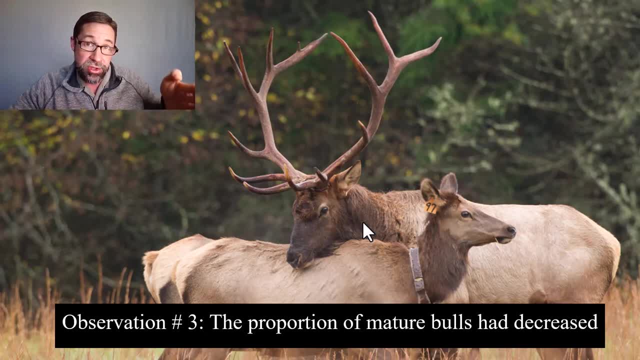 it takes 22 days before she'll release another egg. So what could happen is, if you don't have enough mature bulls, that rut can suddenly be strung out over a long period of time, which then means the subsequent calving period is strung out over a long period of time And then the total 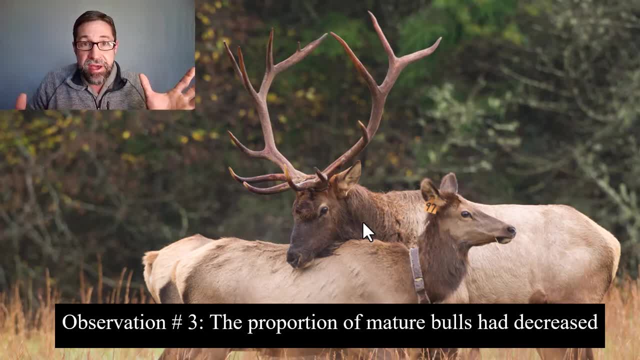 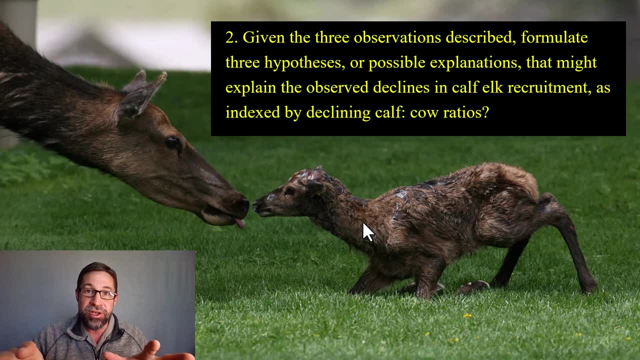 net effect of predation may be considerably greater. All right, so I know I threw a lot at you, but given the three observations that I just described- increasing predator populations, increasing elk densities and decreasing mature bulls- formulate three hypotheses Remember. 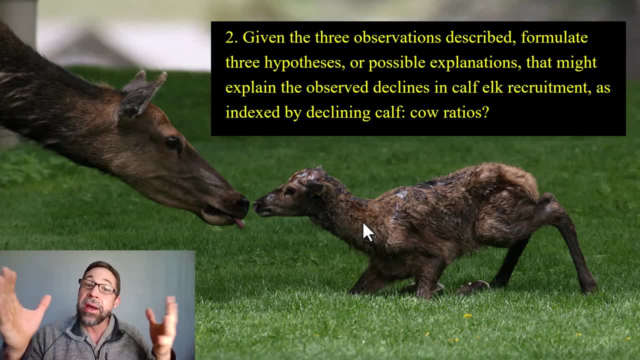 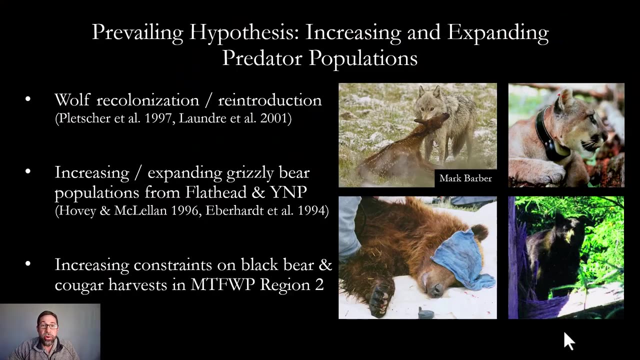 a hypothesis is just a possible explanation that might explain the observed declines that we were witnessing in calf-elk recruitment, as indexed by declining calf-cow ratios. So I'd like to take a moment and point out that when I started this project, the prevailing 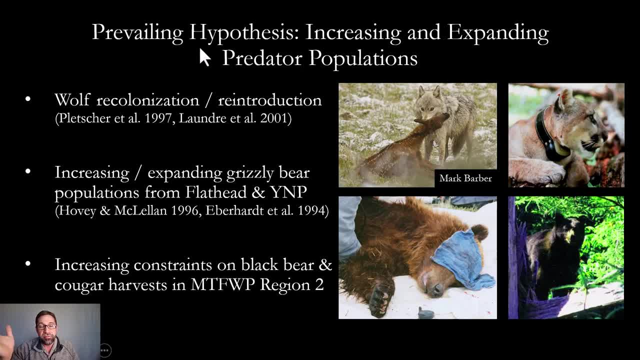 prevailing hypothesis among most wildlife managers and our research team was that it was most likely predators that were exerting top-down influence in regulating this elk herd. That was certainly what they were witnessing just across the state border over in northern Idaho And, as I've mentioned, my advisor, Dr Dan Pletcher, and his students have been doing a lot of research on. 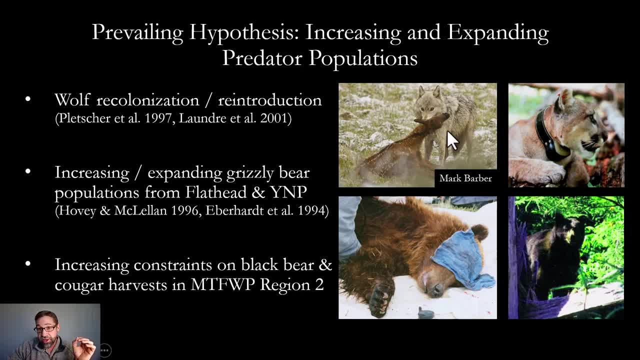 this issue and our students had already documented that wolves had recolonized the area. We knew that mountain lion harvests were suppressed because Montana Fish, Wildlife and Parks had restricted lion harvest And, I should note on my study site, mountain lion harvest had been completely shut down. 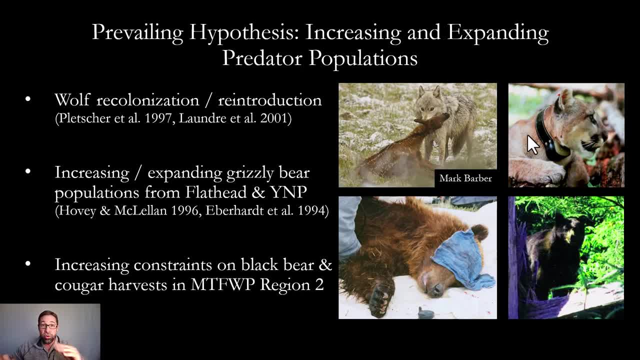 in an attempt to allow those cats to rebound, as well as multiple population estimates, and so I've taken a look at some of the data that I've found to be quite significant. The first thing that I've population estimates of expanding grizzly and black bears, So we know that these predators 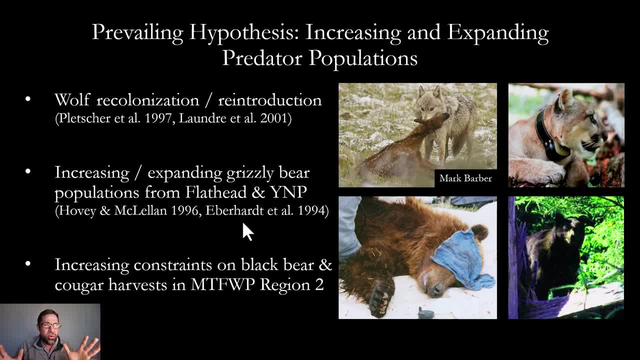 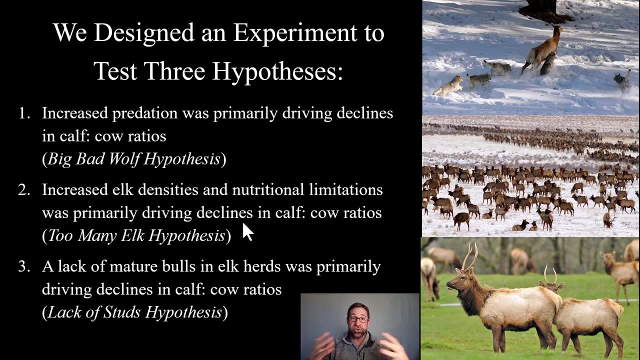 were increasing, but were they the culprits? So this is why we do science, This is why you got to get out and do the field work. So we sought to test not just increased predation but a suite of hypotheses systematically. We used what's called the hypothetico-deductive method. 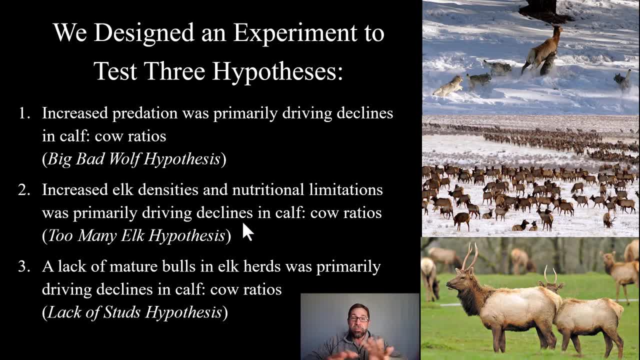 which I'll cover here shortly. But essentially we put forth several hypotheses in an attempt to explain declining recruitment and then sought to design an experiment, our experimental design, to knock those hypotheses down, to disprove them. Okay, the first that we tested was obviously: 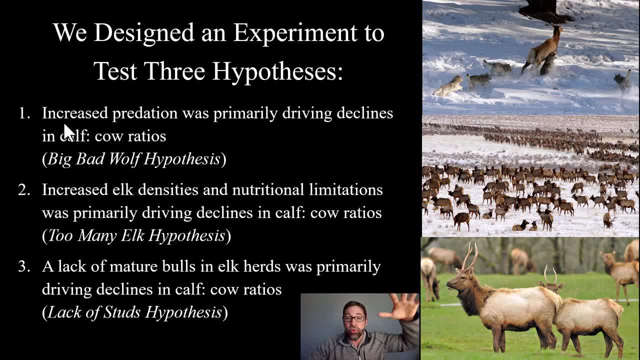 individualized. So we got to get out and do the field work, So we got to get out and do the experimental design to knock those hypotheses down, to disprove them. Okay, the first that we increased predation: perhaps elk herds were being regulated from the top down and predators were. 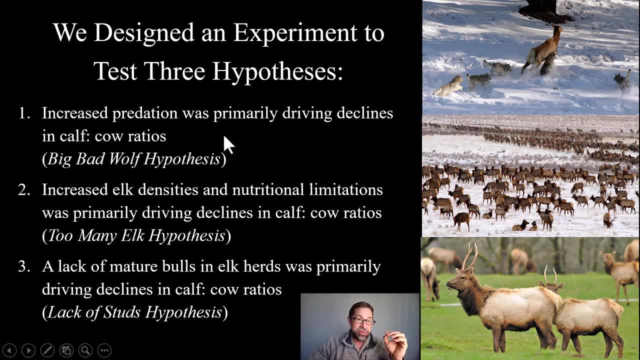 suppressing calf, elk survival and recruitment, which I call the big bad wolf hypothesis, Although it's more, maybe more than just wolves. The second hypothesis that we tested was: perhaps this was an example of bottom-up regulation. We know that elk exhibit density-dependent logistic growth, So 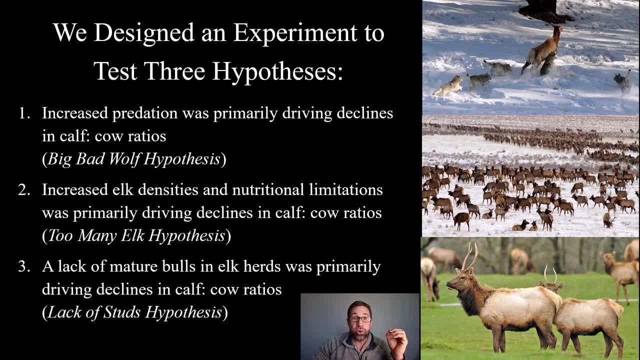 perhaps growth rates were slowing and this elk herd was reaching its ecological carrying capacity and these increased densities were manifesting as decreased pregnancy rates and or decreased survival in these calves, which was suppressing recruitment. We call this the too many elk hypothesis. And then the third hypothesis that we sought to explicitly test was: maybe it was a lack. of mature bulls because of the harvest regime of the previous decades. Maybe there weren't enough mature bulls in the system and spike bulls were doing most of the breeding, which resulted in an asynchronous rut and then an asynchronous calving period in the spring, resulting in greater net. 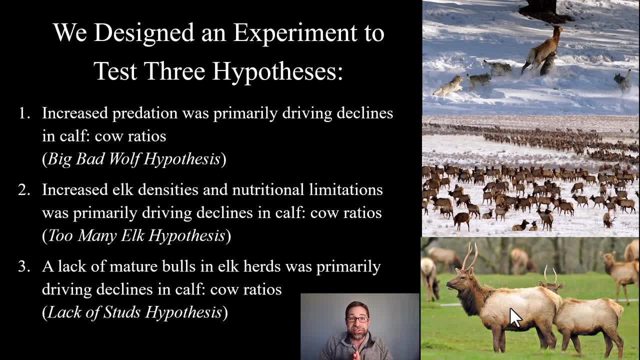 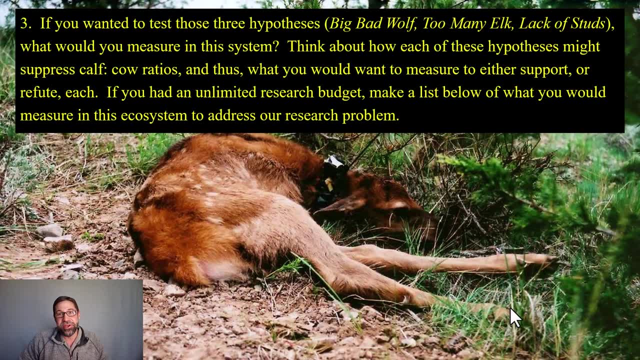 predation rates. Okay, so three hypotheses that we sought to test in our experimental design. If you wanted to test those three hypotheses, what would you measure in the system? So think about how each of those hypotheses- the big bad wolf, the too many elk and the lack of studs- might. 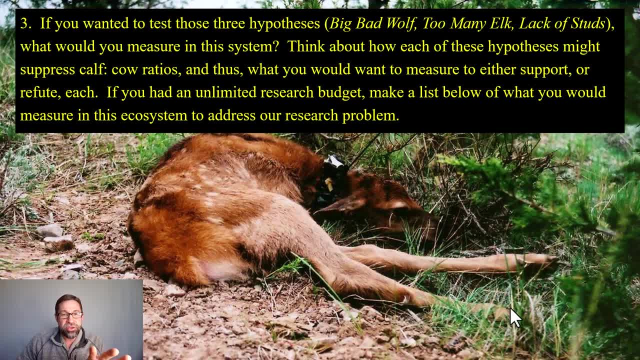 actually suppress calf-cow ratios mechanistically? How might they actually be doing it? Okay, and as such, what would you measure to either support or refute each of these? So pretend like you had an unlimited research budget, which that certainly wasn't the case with us, but money is no. 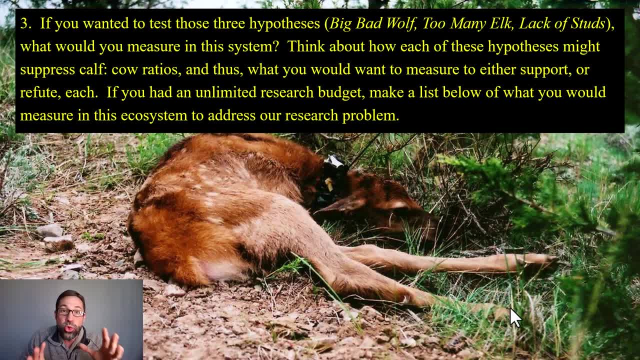 object: Make a list of what you would measure in this ecosystem in order to test these three hypotheses, And it's okay if you don't come up with the same list that we did. That's okay. I just want you to think through this like a scientist. 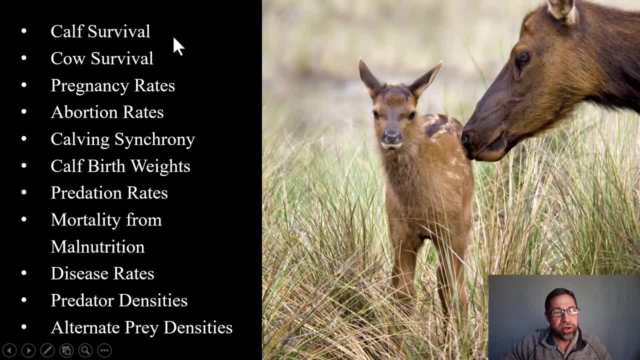 All right. so what did we select to measure? So give me a few examples. Given our budgetary constraints, we measured all of these things in an attempt to test those three hypotheses. It was a pretty ambitious game plan. First and foremost, we needed to get at calf survival. We needed to know what proportion of these newborn calves were actually surviving. 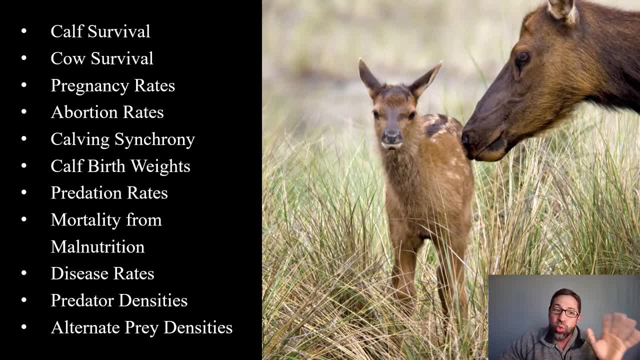 We needed to estimate calf survival rate as well as cause-specific mortality rates, The ones that were dying. were they dying from predation? Were they dying from malnutrition disease? we also radio marked cows to estimate their survival and to assess pregnancy rates. so we did this in two ways. one, by looking at the blood serum. 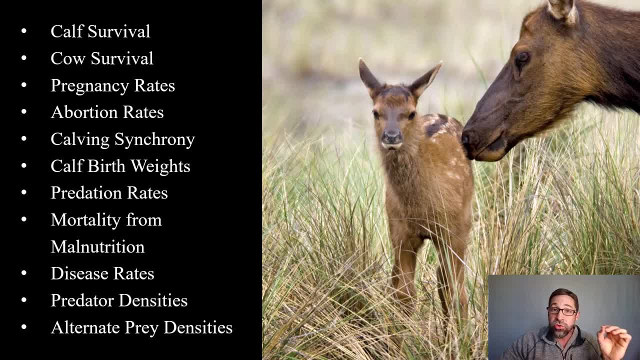 of radio marked cows and then also by sampling fecal progesterone levels. so we would in late winter spend hours watching cows and then collect fresh fecal samples to determine the level of progesterone metabolites, to determine pregnancy rates. in that way we estimated abortion rates as best we could, by 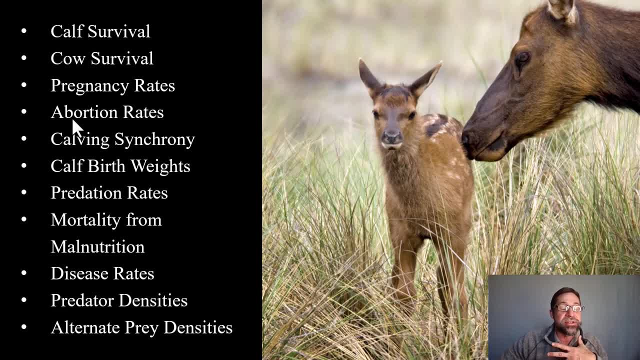 tracking known cows known to be pregnant to determine if they carried their calf to term. we looked at calving synchrony. this was really important. were those calves really all hitting the ground in a short period of time in the late spring in a very synchronized calving period, or was 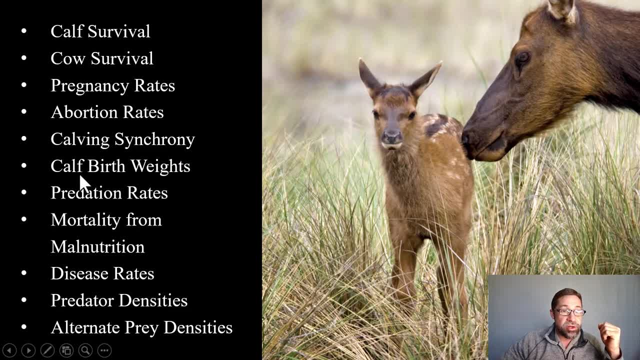 calving synchrony in the late spring or was calving synchrony in the late spring calving strung out? Fortunately, we looked at calf birth weights and this turns out to be really important. How heavy were those calves when they were born and did that fluctuate?